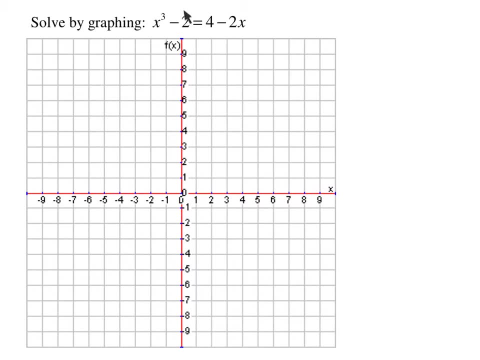 Alrighty, if I want to solve this by graphing, what I'm going to do is: I'm going to graph this side: It is y equals x cubed minus 2.. And I'm also going to graph this side, which is y equals 4 minus 2x a line. 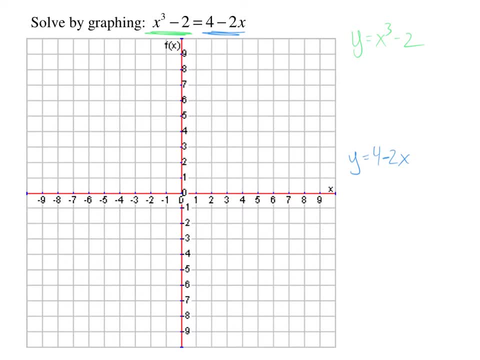 So if I graph both of these to solve it, I'm looking where they cross. Now to graph this, let me show you something to clarify this a little bit. Let me put it the AHK format. So I'm going to change this to look like this: 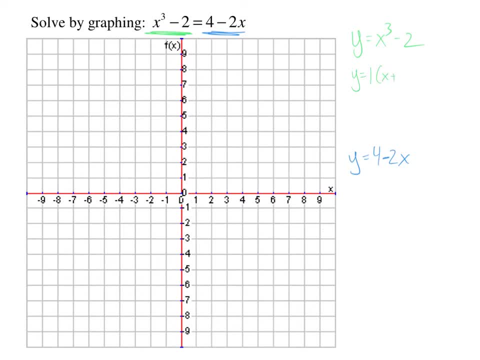 This is really 1x plus nothing, cubed minus 2.. Do I have to write that second formula? No, but it might help you graph. For some of you, this right here is more familiar for graphing than this one. It's your call. 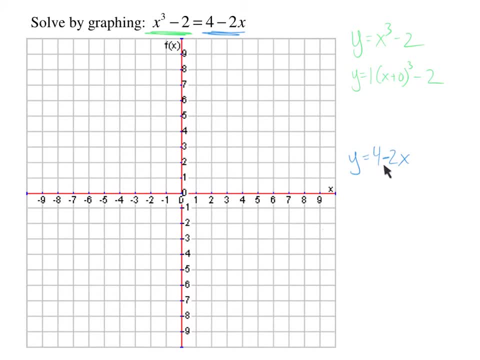 You could totally graph this one, if you can make sense of it. This is a line. This is more straightforward. So let's graph this and let's graph this. So this one. what is my HK for this one? Well, it's 0, negative 2.. 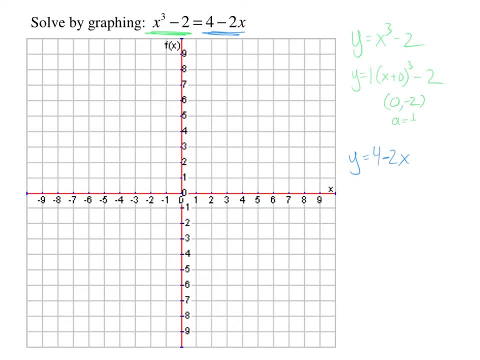 My A value is 1, which is a positive, So let's graph it. We are going to put a 0 at 0.. Sorry, we're going to put a vertex or a HK, at 0, negative 2.. 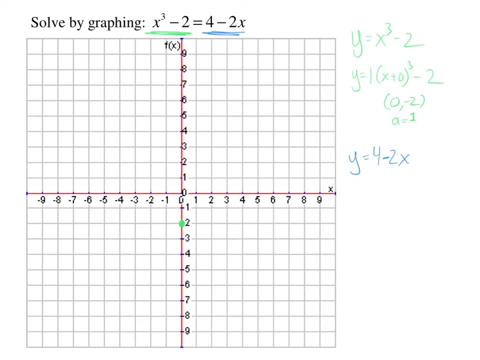 Got it right there: 0, negative 2 right here, And this is a cubic. What's a cubic mean? If it's a positive A and it's cubic, doesn't that mean it's going to go up like this and down the other direction? 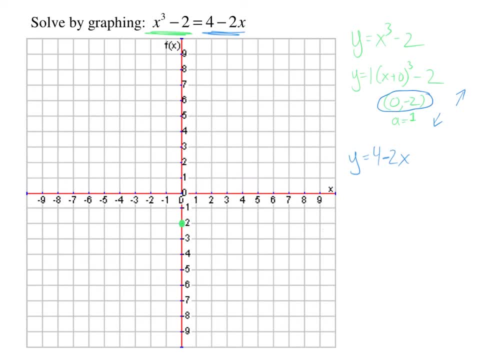 So isn't it going to twist right here? Isn't there going to be a twist right there at 0, negative 2?? So what's going to happen is, at this point I'm going to go right 1 and up 1, because my A is 1.. 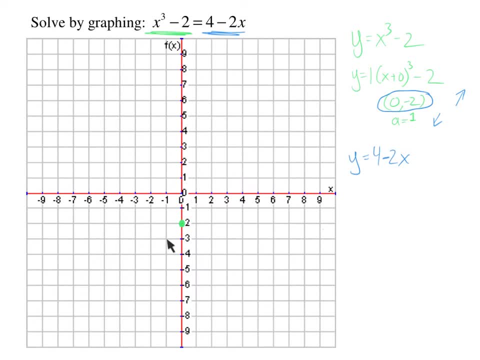 And I'm going to go. I'm going to go this way and down 1, because my A is 1. And that's going to have my little twisty look. So I'm going to put a dot here And it's going to look something like that: 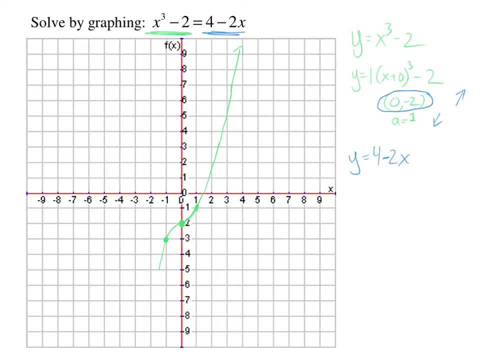 And over here we're going to twist and hit right there. It's not a perfect sketch, but we've got the basic look of it. We can tell this one's going to go like that and this one's going to go like that.